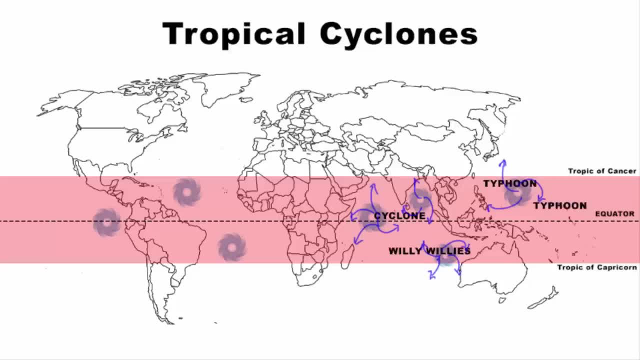 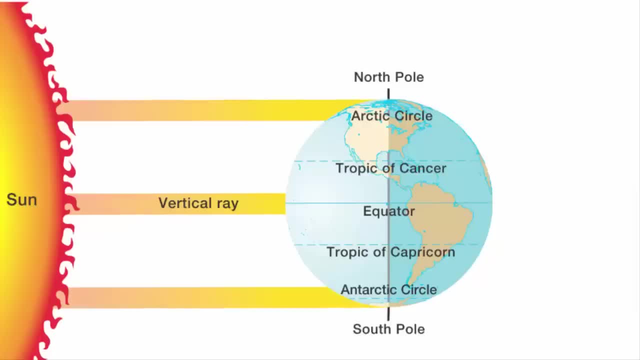 Likewise, near Western Australia, it is known by willy-willies- All these are different names referred to the same type of storm. You must be knowing this: that tropical region receives the most solar radiation per area and the reason behind that is due to the incoming solar radiation. 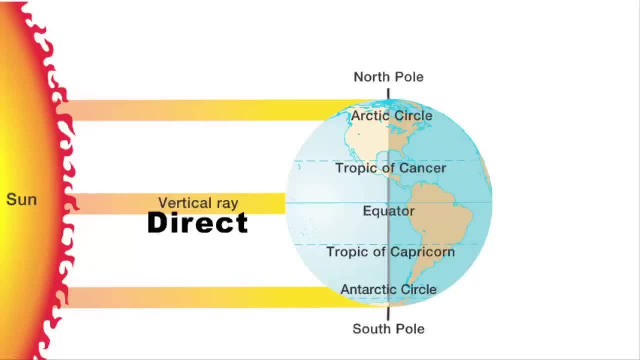 you must be knowing this: that tropical region receives the most solar radiation per area and the reason behind that is due to the incoming solar radiation that are direct and vertical. at the tropical region and as you move towards the polar region, the angle of the Sun rays are not vertical, they are 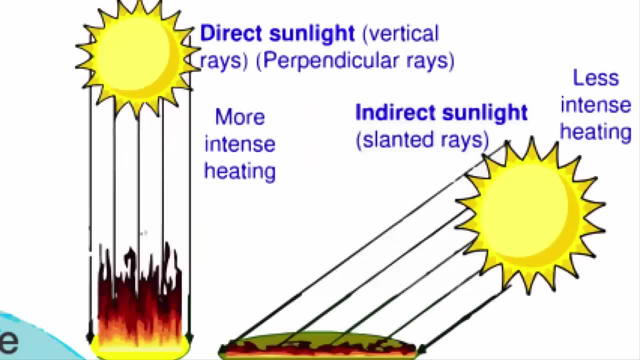 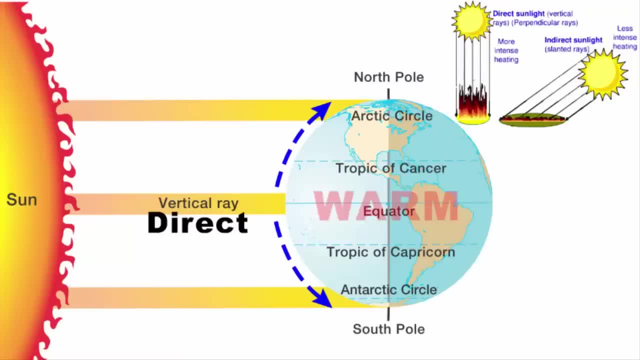 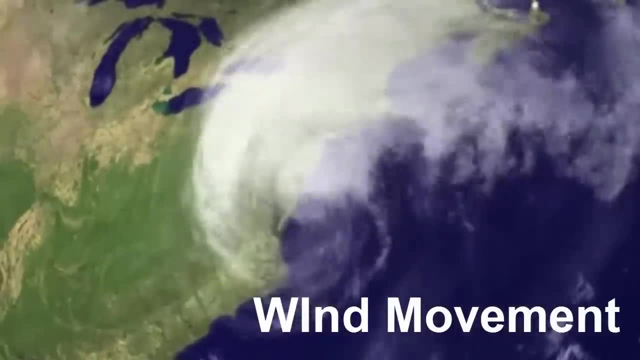 slanting rays. Vertical rays of sunlight are more effective in producing light and heat than slanting rays, and that's why the tropical region is warm. Now that you have understood the main things about the tropical region, let's understand about wind movement. Wind movement is determined by the 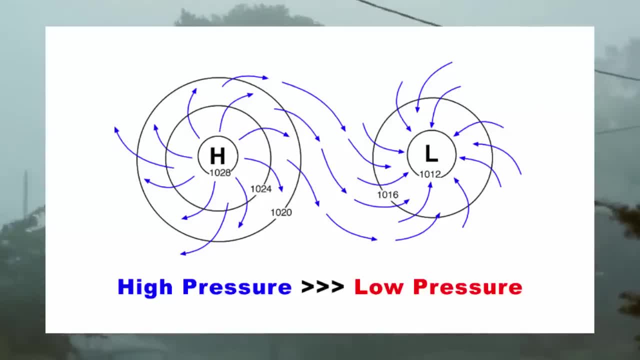 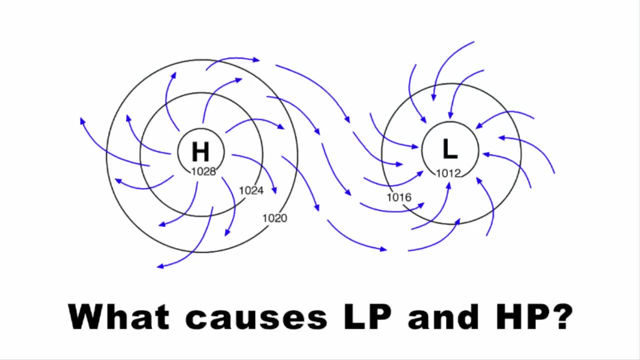 low pressure and high pressure systems. It is the differences in atmospheric pressure that creates pressure gradient and makes the wind move, and wind always blow from the areas of high pressure to low pressure areas. Now the next question is: what causes low pressure and high pressure? Low pressure occurs when air is 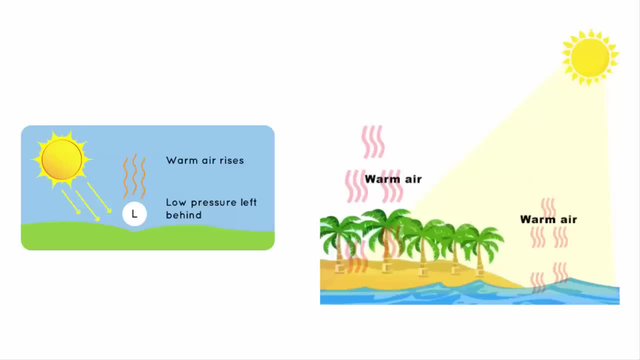 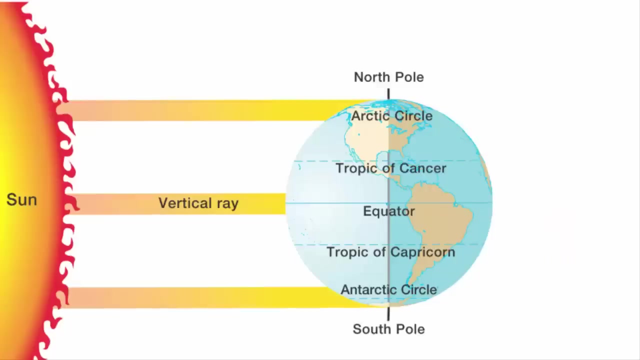 warm either from being over a warm land or ocean surface. That means low pressure occurs at a place which is warm. And how does a place become warm? because of the incoming heat from the Sun. That is why tropical region is a perfect place where low pressure occurs. Similarly, 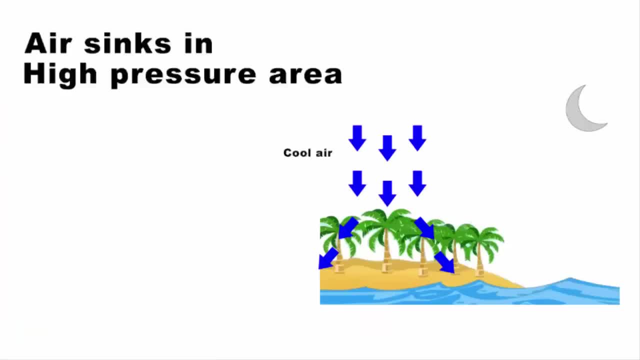 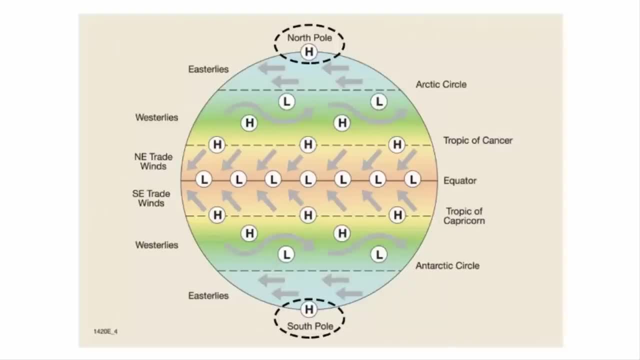 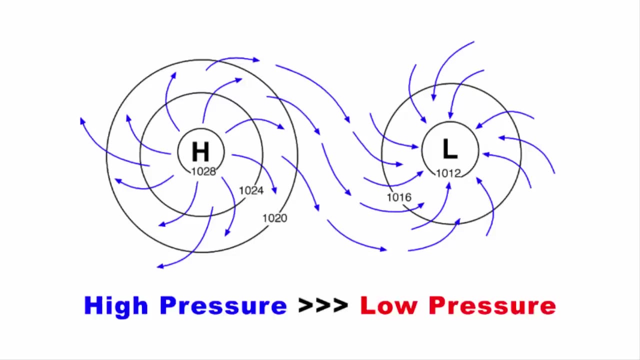 high pressure occurs when air is cool, either from being over a cool land or ocean surface. That is why in the polar region, that is, your north and south pole, it is a high pressure zone and always remember, winds blow from the areas of high pressure to low pressure areas. 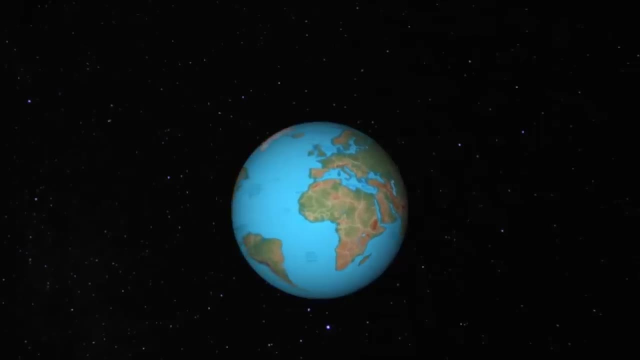 While all of this happens, there's another important phenomena which comes into the picture. It's called Coriolis force. Due to the rotation of the earth, the earth rotates towards the east, and that's why the Sun, moon, planets and stars all rise in the east and go towards the west. 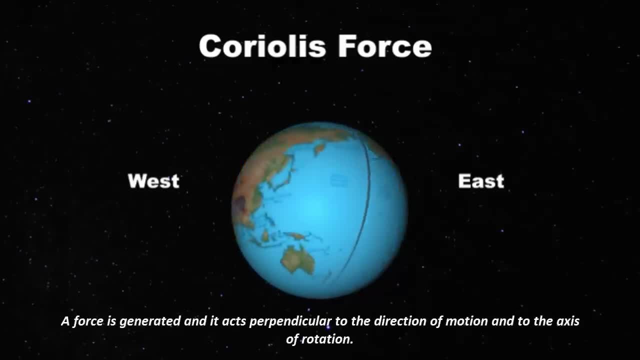 Anyways, due to the rotation of the earth, there is a force that is generated and it acts perpendicular to the direction of motion and to the axis of rotation. In simple terms, when the earth is spinning in its axis from west to east- and we also know that earth is a sphere and it is much wider in the middle- As a 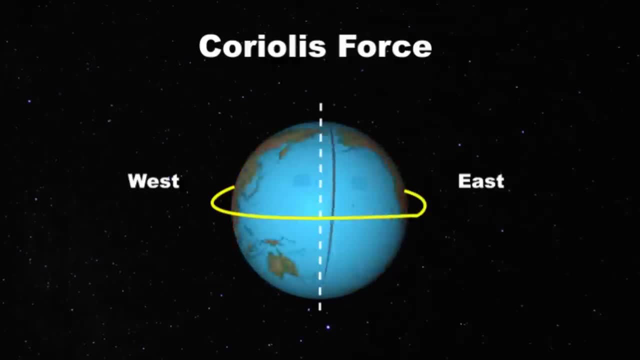 result, the speed of the surface of the earth at the equator is much faster than the speed at the poles. So if anything has to come straight from the poles towards the equator, it gets deflected to the right in the northern hemisphere and to the left in the southern hemisphere. 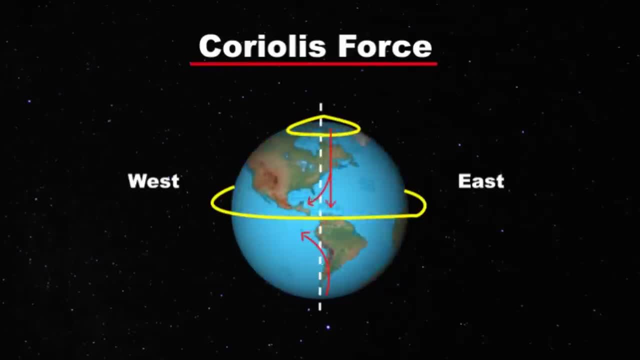 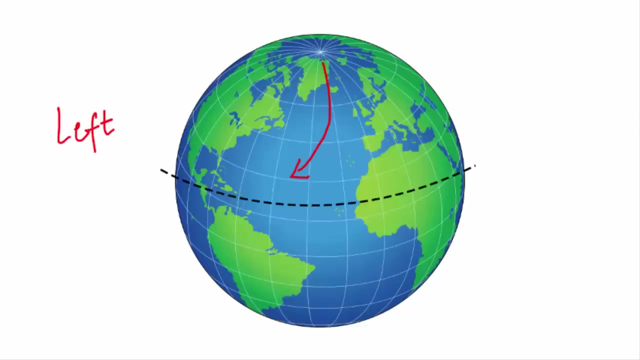 And this force that we are talking about is called Coriolis force. It causes fluids like water and air to curve as they travel across or above the earth's surface. Due to Coriolis force, the air in the northern hemisphere gets deflected to the right side. Now you might think, no, that is going towards the left side, but 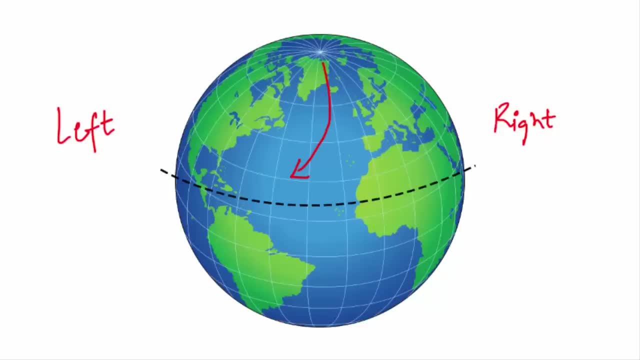 then I said the air is going to curve to the right side in the northern hemisphere. To clear your confusion, you have to actually see it from the direction in which the wind is moving. So what I'm going to do is I'm going to rotate this picture and now put yourself in the path. 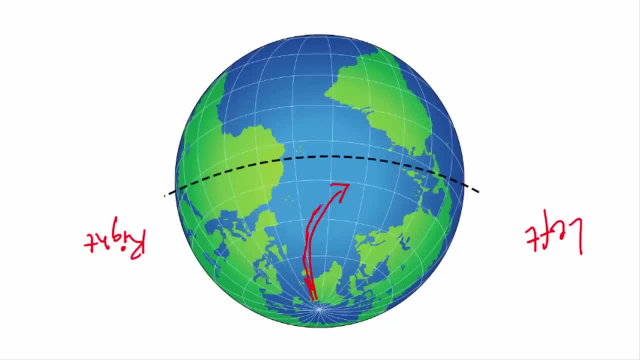 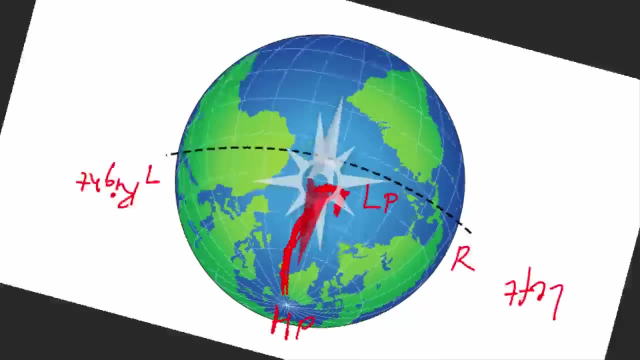 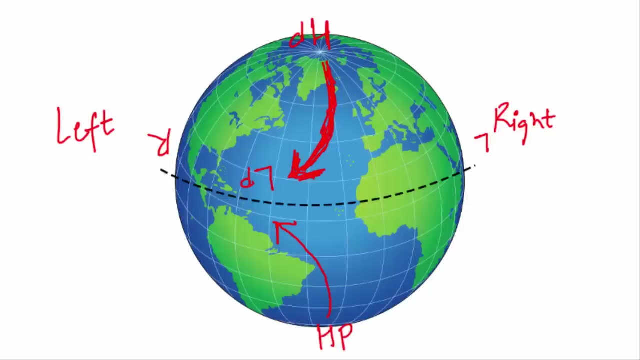 of the wind. Now you will be able to see that the air in the northern hemisphere curves to the right, while moving from high pressure to the low pressure area. Similarly, in the southern hemisphere, the air is deflected to the left side, while moving from high pressure to low pressure area. In this case, we don't have 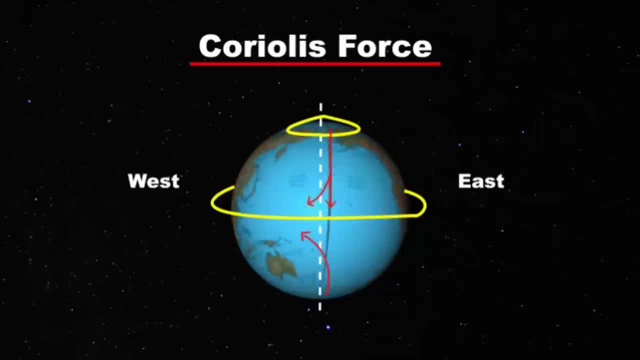 to rotate the picture. Now that you have understood why the air moves to the left and right due to Coriolis force, just remember this point: that it is because of this reason there are certain pressure belts all over the earth's surface You must be familiar with. 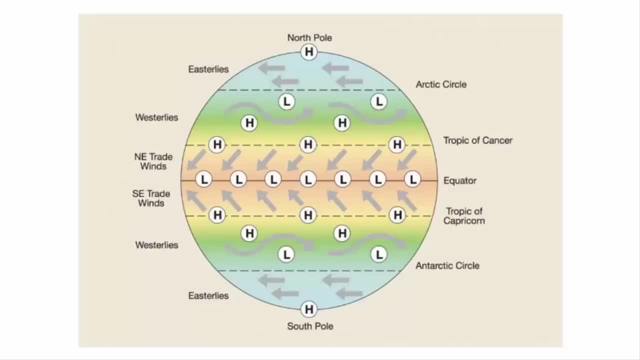 this picture, which shows global wind circulation pattern. You can see that at different latitudes there are different pressure belts. Their existence is simply due to the movement of air to the left and right, due to Coriolis force. I hope so far you have understood the general movement of air. Now let's